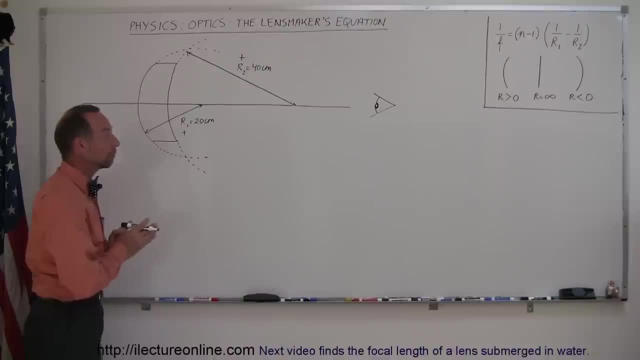 Welcome to Electron Line. Here's example number two of how to find the focal length of a lens, And so we're going to use the lens maker's equation. Again, n is the index of refraction of the lens, And let's assume that this is equal to 1.5.. The lens is immersed in air, So 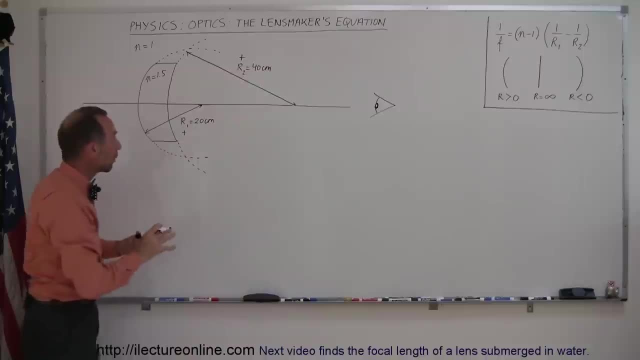 n equals 1 is the index of refraction of the medium around the lens. The radius of curvature of the front side of the lens is 20 centimeters. The radius of curvature of the back side of the lens- you can see it doesn't curve as much- is therefore longer, And here it's 40 centimeters. 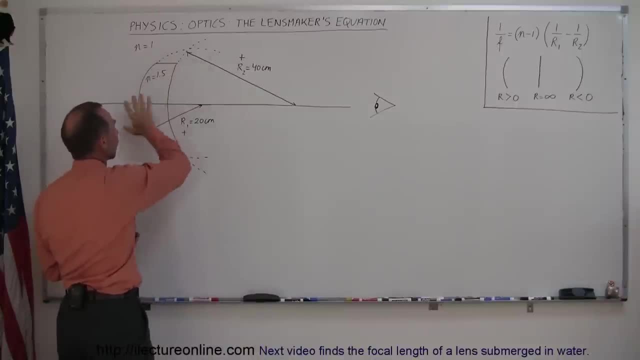 Notice that both cases, the front and the back side of the lens curve away from the observer. And when it curves away from the observer we call the radius of curvature positive. All right, Writing down the lens maker's equation, we have: 1 over f is equal to the index of refraction. 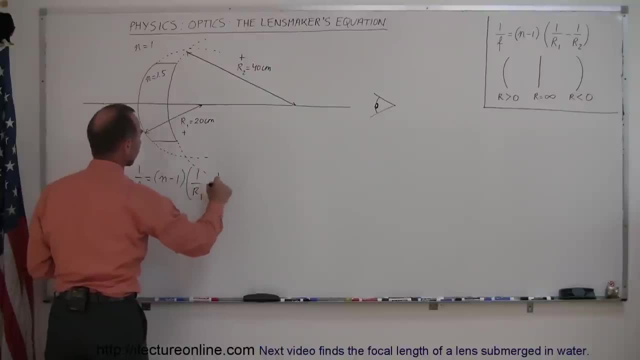 of the lens minus 1 times 1 over r1, minus 1 over r2.. Plugging in numbers we have 1 over f is equal to the index of refraction of the lens minus 1 times r1, minus 1 over r2.. 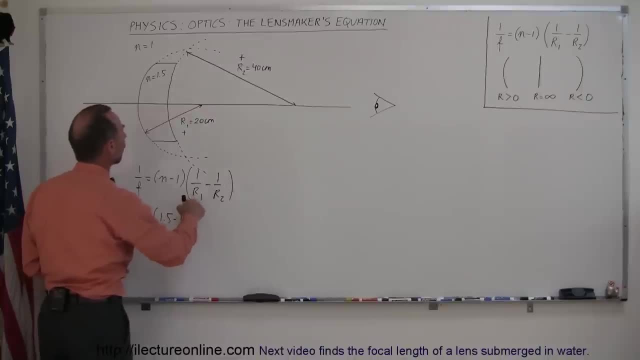 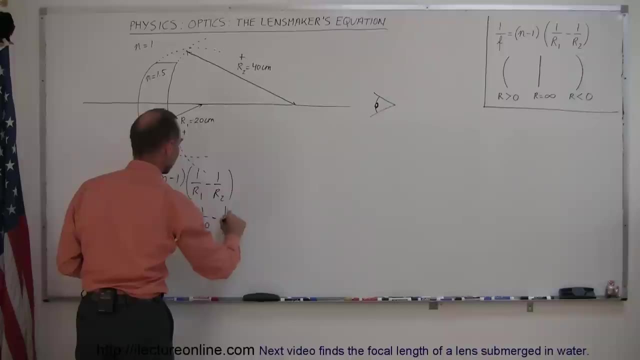 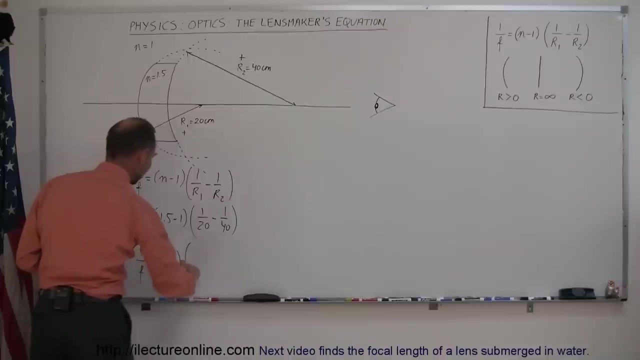 to 1.5 minus 1 times 1 over r1. r1 is a positive 20 centimeters minus 1 over r2 and r2 is a positive 40 centimeters. okay, so simplifying this, we have: 1 over f is equal to 0.5 times. now we need a common 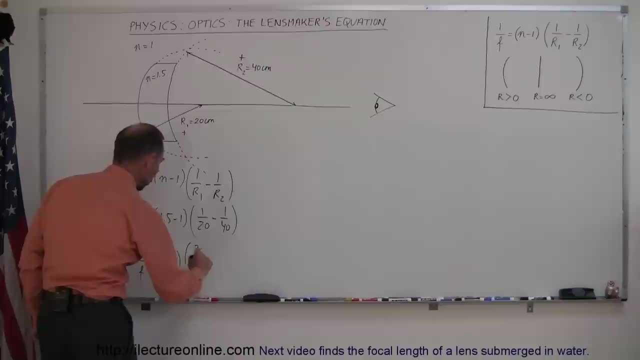 denominator here. so i'm going to make that 40, so we have 2 over 40 minus 1 over 40, and then continuing on over here, so we have the focal length equals 0.5 or 1 over the focal length equals 0.5 times and, of course, 2 over 40 minus 1 over 40 is 1 over 40. 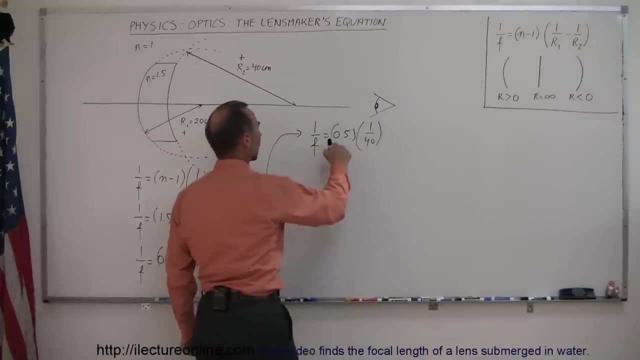 so now we can multiply that together, we have: 1 over f is equal to 0.5 over 40. now turning the equation around, because we're looking for f, not 1 over f. so f is equal to 40 over 0.5 and, of course, 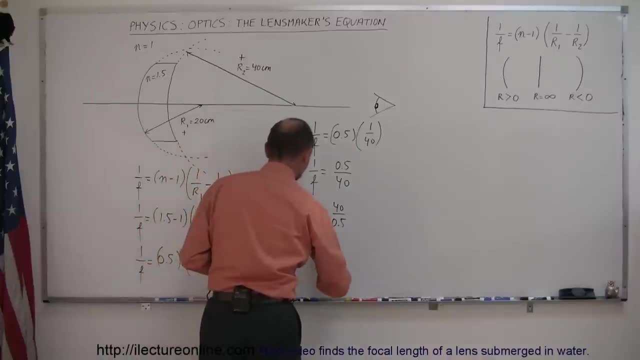 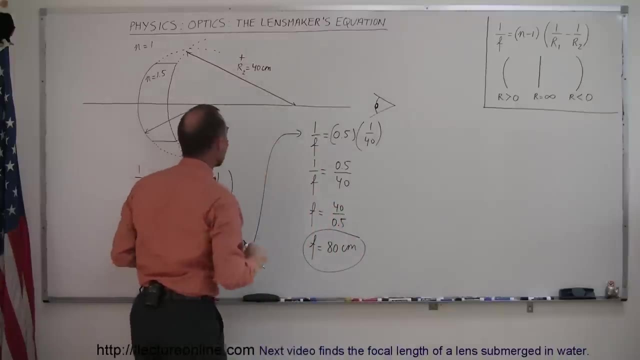 divided by half is the same. it's like multiplication multiplying times two, and so the focal length of this lens is equal to 80, and it will use centimeters, because we use centimeters for the radii of curvature of the both sides of the lens.